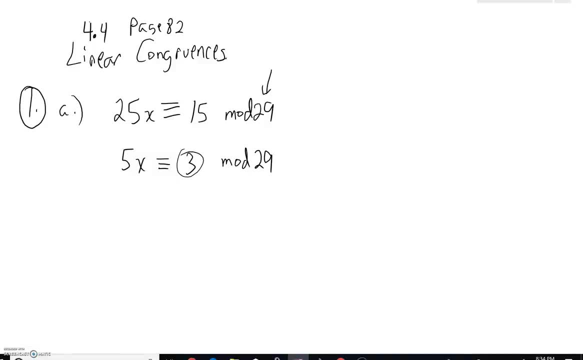 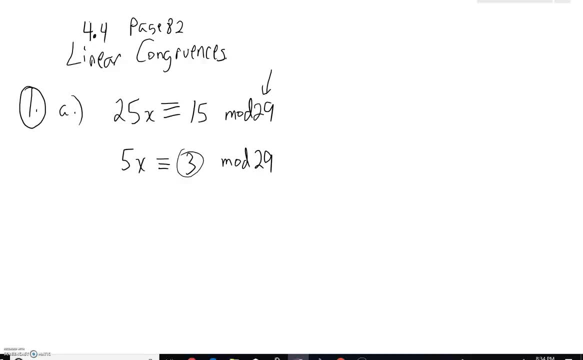 I think a lot of times students avoid working with negatives. but we certainly could Look if we subtracted 3 minus 29,. you know, of course we would get a negative 26.. If we'd subtract 29 yet again, I think you could see you'd get negative 55.. 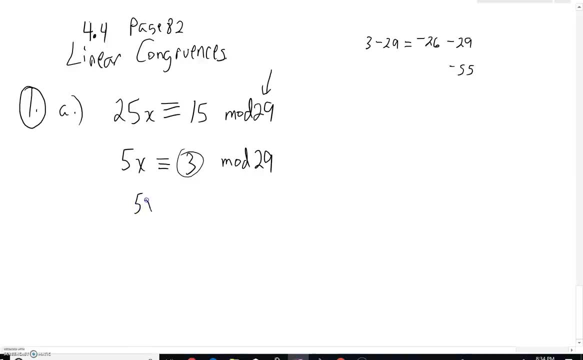 Now, if you were to do that, by the way, you certainly could do that. Now, if you were to do that, by the way, you certainly could do that- You might wonder why I can look at that 3 by adding or subtracting an appropriate number of 29s here. 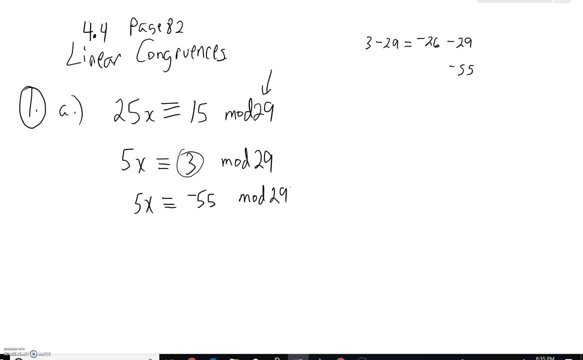 because I might just find a friendly multiple of 5, and I have. I'm going to divide both sides by 5 right now, And again I don't have to worry about changing my mod. And hey, look at that Right now you can see that we've got 29.. 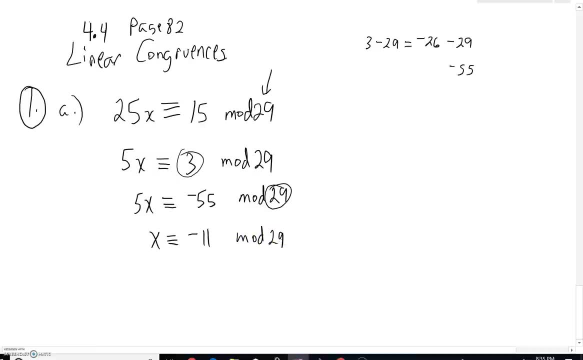 And hey, look at that Right now, you can see that we've got 29.. And hey, look at that Right now, you can see that we've got 29.. x is congruent to negative 11 mod 29.. 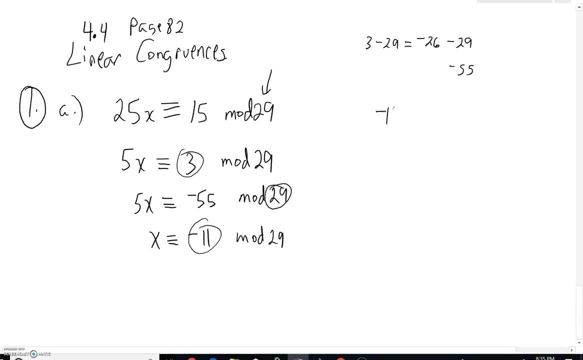 And then, of course, you could think: well, is that a legitimate answer? Well, of course you know. I'll tell you what, though, If we added 29 to it, we could then write it in a maybe more familiar form. 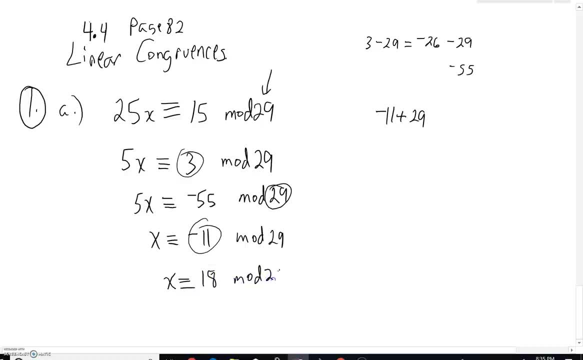 x is congruent to 18 mod 29.. So this is a little bit different measure of solving And it's certainly not the only way There's inspection. There's so many other ways that you can proceed, But you know this is kind of slick. 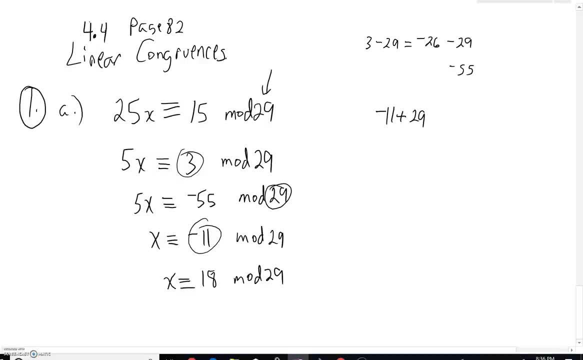 This is kind of cool and I want you to see this Now. by the way, I forgot to address something earlier and I really should have. The greatest common divisor of 25 and 29 is 1.. We were talking about this going over things in the textbook. 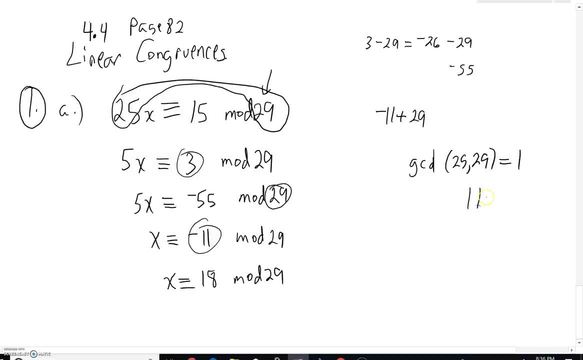 The GCD is 1. And that means also, of course, 1 certainly divides 15.. 1 goes into 15.. So we know, in fact, there will be a unique solution And, in fact, our unique solution. we're going to have one unique solution right here. 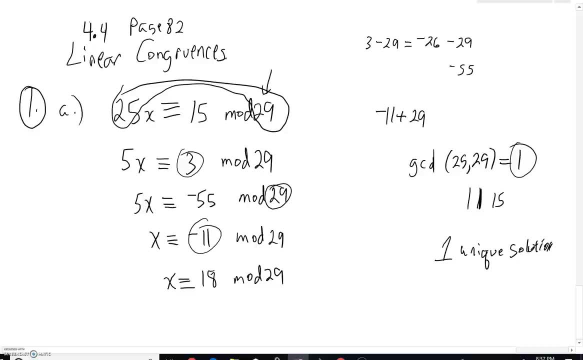 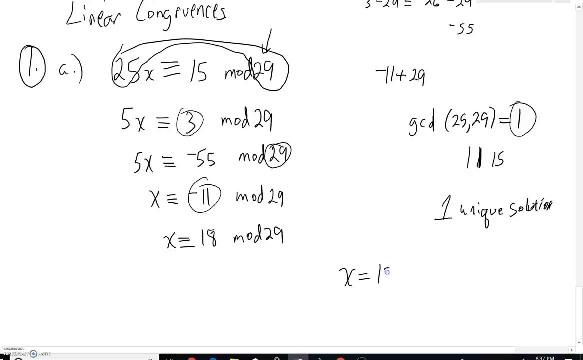 And that's going to be x, is congruent to 18.. Another way we could write this, the way our author was writing it, is to say it's 18.. 18 plus our mod divided by that, you know greatest common divisor here of 1 with a t. 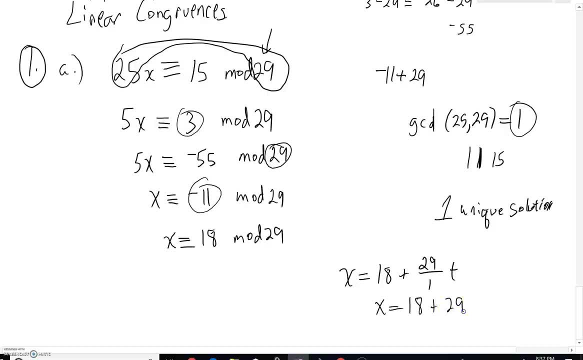 So x would be 18 plus multiples of 29.. You know, here's an alternate way of writing it, But this solution in terms of a mod would be just as good too. Of course we'd have: x is congruent to 18, mod 29.. 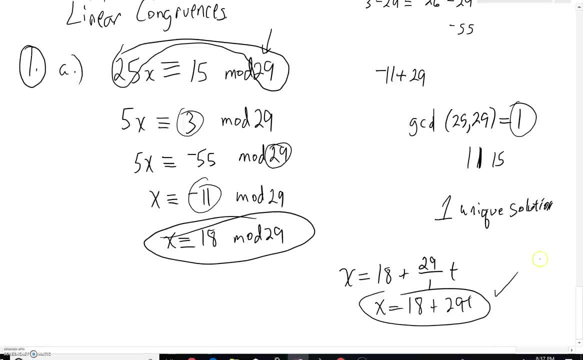 Why do we write it really parametrically like this: x equals 18 plus 29t. That's, of course, if you'd like to generate more answers, Very often you might have more than one solution. So let me flip back over here in our book. 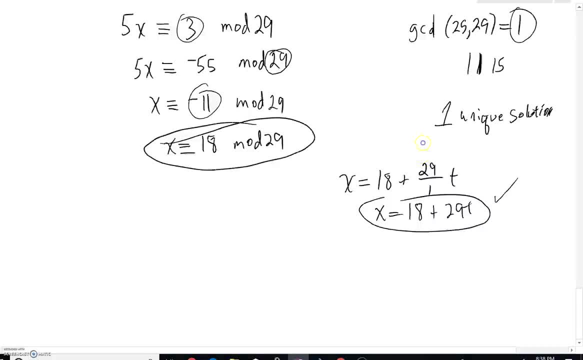 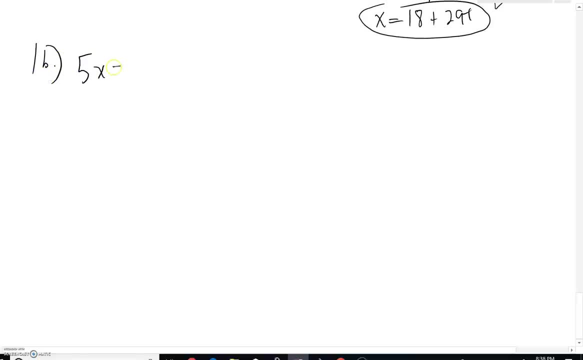 I guess we have for b. maybe we can go to 1b here and just keep going. I think this can be helpful to look at some of these problems. 5x is congruent to 2. Mod 29. 26. 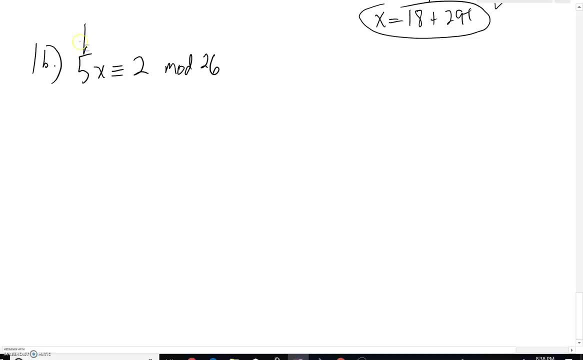 And again, maybe we should check and see if there is an answer. By the way, that's very important. My goodness, you can save yourself a whole lot of work if you quickly realize there wouldn't be a solution. Greatest common divisor of 5 and 26 is 1.. 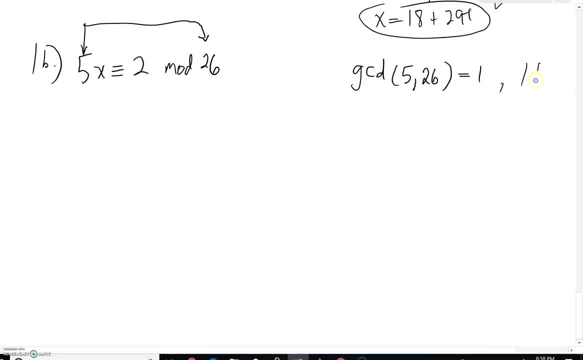 I'll tell you what. you know that 1 is going to divide anything. It certainly divides the 2.. So there is one solution here. There's going to be A definite answer. So, right here, we're not going to start by dividing things. 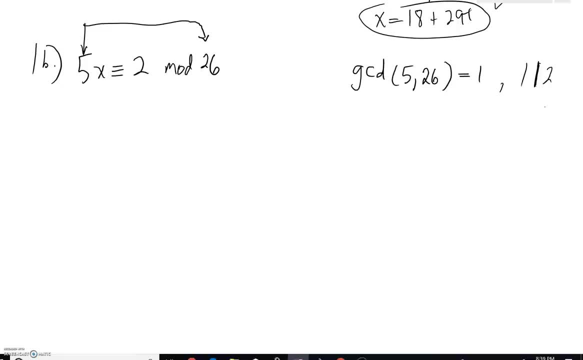 But you know, maybe we could piggyback on what we just did a moment ago. You could think: hey, could we perhaps add multiples of 26 or subtract multiples of 26 here? And you know, honestly, you could go either route. 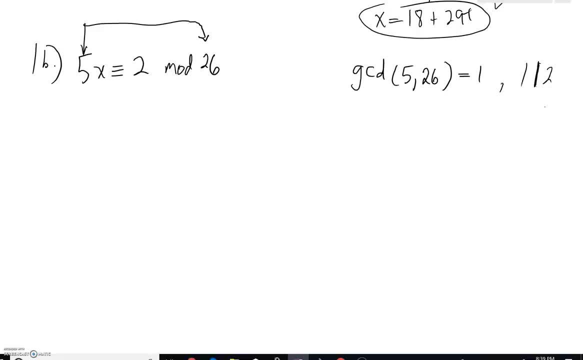 You certainly could do that. You're looking for a multiple of 5.. You know, kids can really run away from that negative idea And maybe we should see if we can do that again. Let's see if we can. I think we can just previewing. 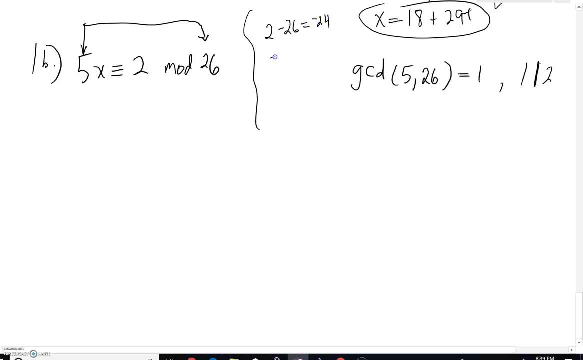 You know, 2 minus 26, you'd get negative 24.. And if you subtracted 26 again- I saw that 6 and 4 coming up in my head- you'd get negative 50. So the 2, you could say: well, what is 2 equivalent to? 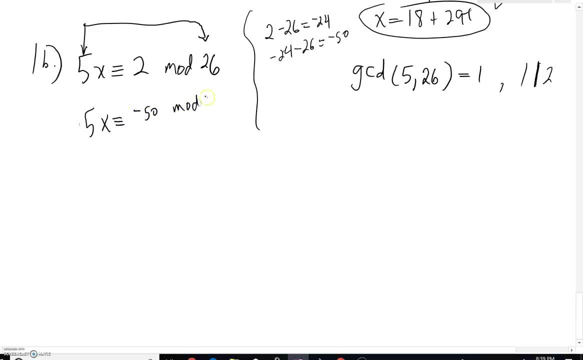 Wow, it's equivalent To negative 50.. And sometimes kids look at that and they'll say: I don't know about that, But look, if we just did a whole separate problem here. a bold claim. could 2 really be the same thing as negative 50 in mod 26?? 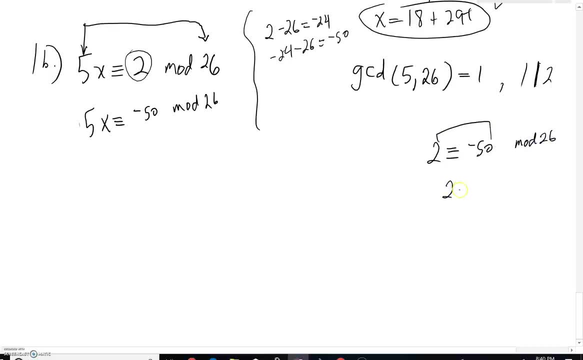 A lot of times kids will say: I don't know if that's true. Well, remember, we'd say: if you subtract these two, well let's see: 2 minus negative 50 is positive 52. If 26 divides that, well, albeit it does. 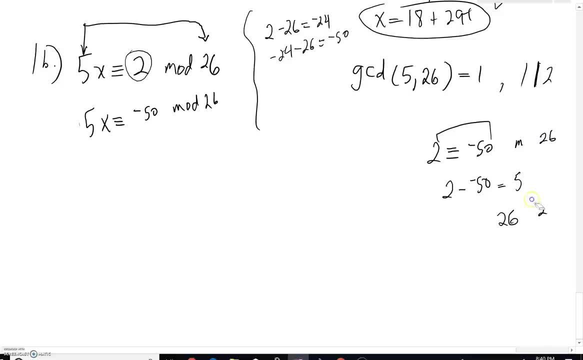 Look at that: 52 is a multiple of 26.. So you know what you're doing is valid. You know, could we have continued to add 26 until we get a nice multiple of 5?? Well, yeah, You could do that too. 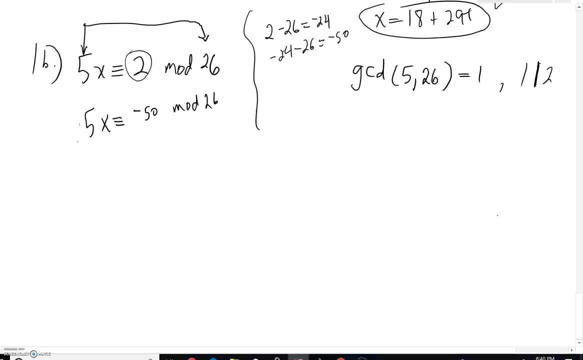 Dividing by 5 right now. well, my goodness, I think you could see that, the left side, you'd get x. Then you'd get what negative 10.. And Here we go, We could just add a 26 to negative 10, and you'd get 15.. 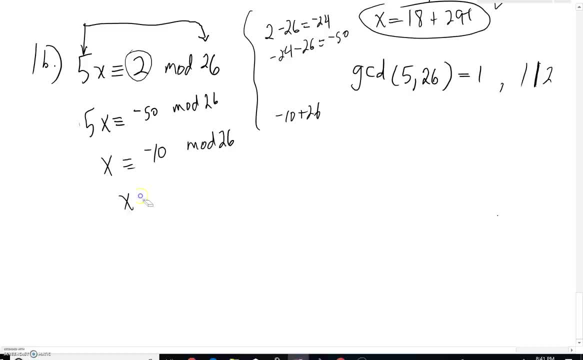 So really, negative, 10 is equivalent to 15.. This is in mod 26. But here we go again. We can say: well, we could write it this way, which is, you know, fine, You know, that's in mod form. 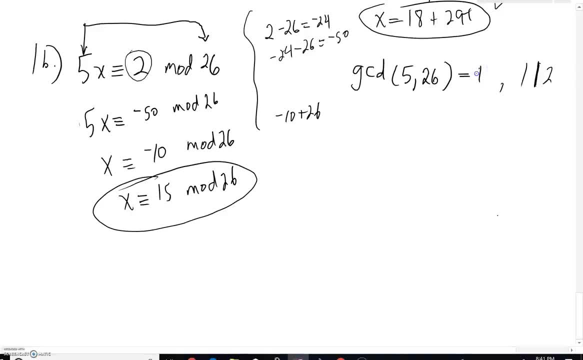 If you would have had multiple answers. you know when your GCD is just a 1, hey, that's great. You know you're just going to have one solution and you just found it. But you might wonder what that solution would look like being written out in a parametric generation. 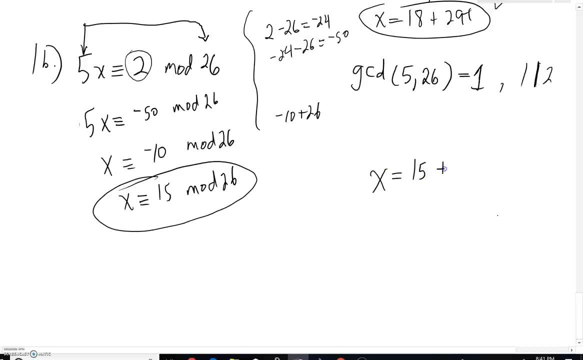 You could say x equals 15 plus and you've got your mod 26 divided by that 1. And you have a t, So you're more or less saying it's 15 plus multiples of 26. It would be an altered way to write that out. 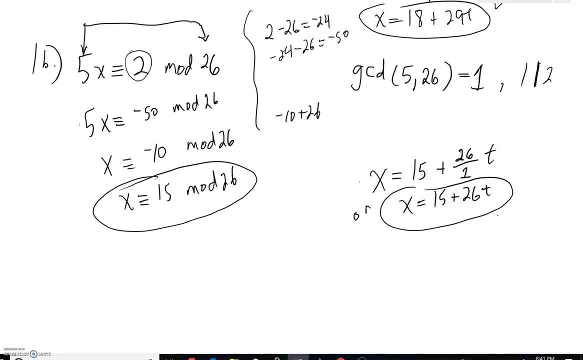 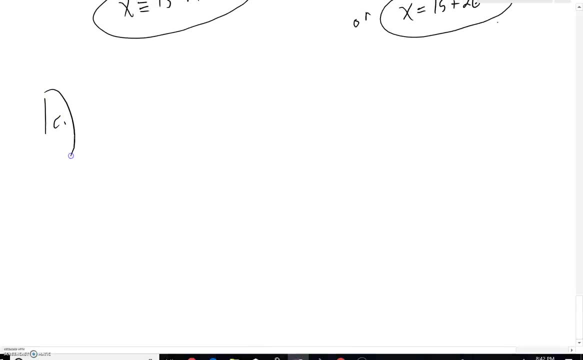 All right. Well, you know, so far we've really lucked out with some of these problems. Let's maybe take a look at 1c, Because I think just looking at that one, that's going to look a little bit more involved. 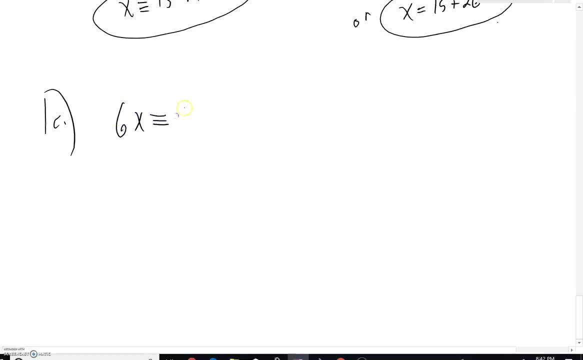 Take a look at this one: 6x is congruent to 15 mod 21.. You know, You know you could divide some things out. for sure You could definitely divide. I think a lot of times kids will say: I want to divide by 3.. 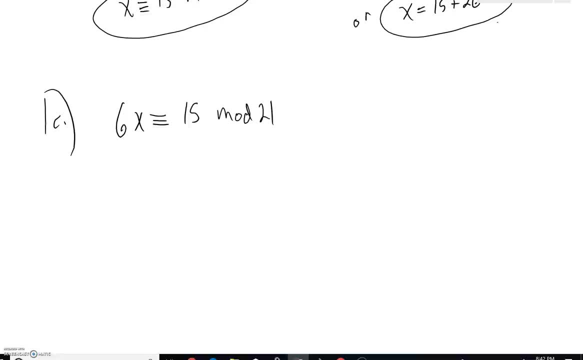 And you can, You definitely can, And you know. maybe we should check and see if there's even an answer. first, You know what's the GCD of 6 and 21?? What's the greatest common divisor that we could ever have? 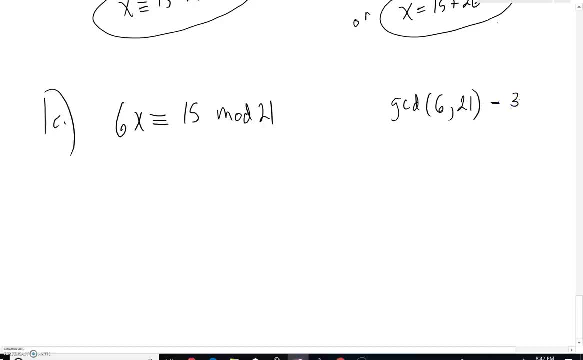 Well, my goodness, it's going to be a 3, isn't it? 3 is the largest number that simultaneously divides 6 and 21.. And 3 divides 15.. So there are 3 solutions here. You know, we've kind of avoided a lot of this. 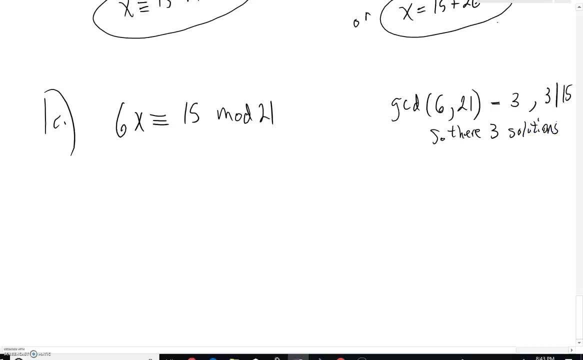 And you know, maybe right now this is a great problem to deal with some of these other issues. I definitely wanted to do a problem like this right now. So look, If we divide this, This congruence, by 3, you could see well, you'd get 2x. 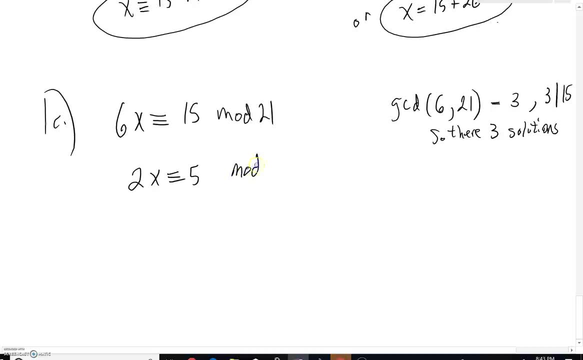 And over here you'd have a 5.. But you have to change your mod, don't you? This is going to be mod 7. now, Right, And you know, could we solve by inspection? Well, of course we could. 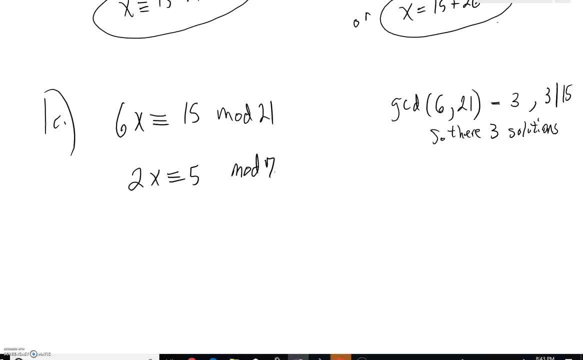 We actually definitely could, And it wouldn't take you too long to be able to find an answer honestly. Eventually, just by doing some guesses And checking and processing and checking, you'd be able to be fine. But I want to show you something really cool too. 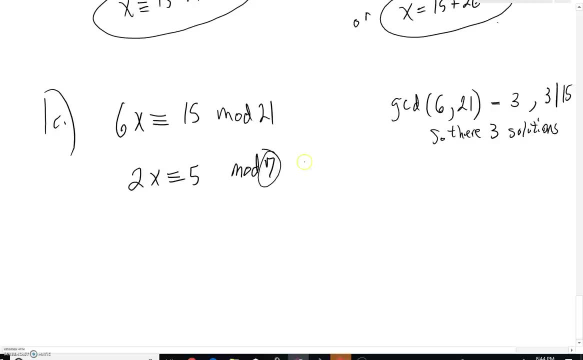 I mean, just like before, we could subtract a 7.. We could add a 7, too. You know, we haven't been adding as much. You could say: well, what's 5 plus 7?? Well, it's 12,, isn't it? 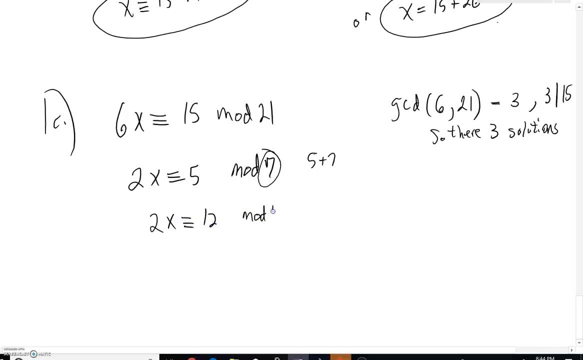 5 right here, would be exactly the same thing as 12 in mod 7.. And then what? Well, right now you can see that you can divide everything by a 2. Look at that. Rather than go by inspection, you might be able to say: hey, there we go. 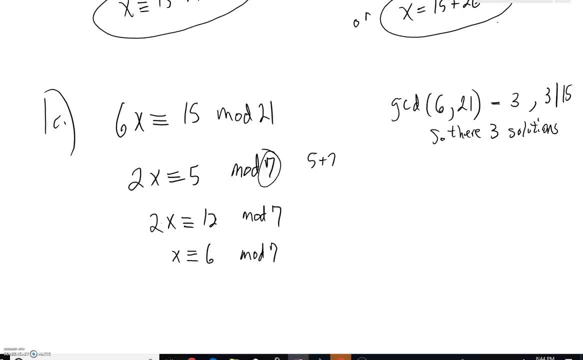 X is going to be congruent to 6.. So that's great, You found an answer. But remember our answers. ultimately, we'd maybe like to go back to mod 21.. So tell you what We can go back to, the way the author was writing this out. 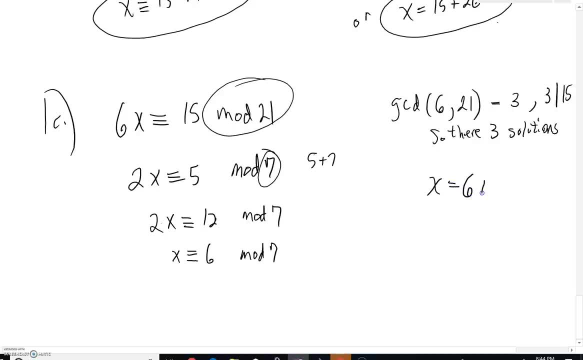 We found a solution That's 6.. But our mod was 21.. This GCD was 6.. This GCD was 3.. And sure enough, would you look at this: 21 divided by 3 is a 7.. 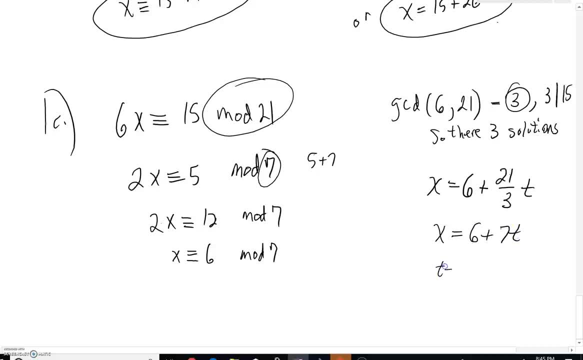 So look, if we had t equal 0,, we'd have x is equal to 6.. If we had t equals 1, we'd have x is equal to 13.. And if t was equal to 2,, well, that's 14 plus 6.. 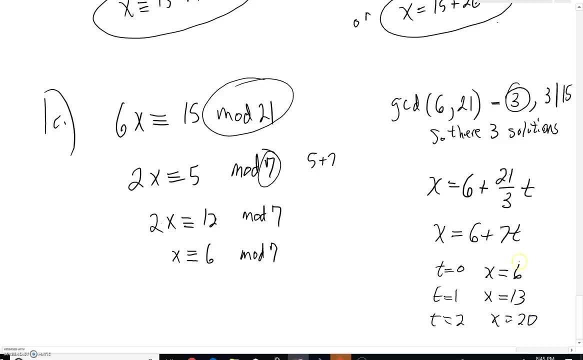 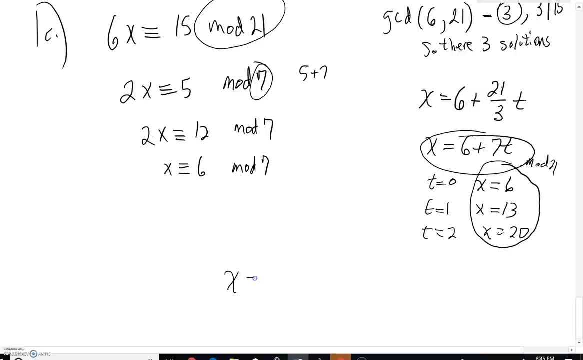 That would be 20,, wouldn't it? So you know, here are three answers. mod 21,. mind you that you could come up from this generator. Now, if you were asked to write it out in terms of a mod, you could say: well, we could say x. well, of course, you could just say x is congruent to 6.. 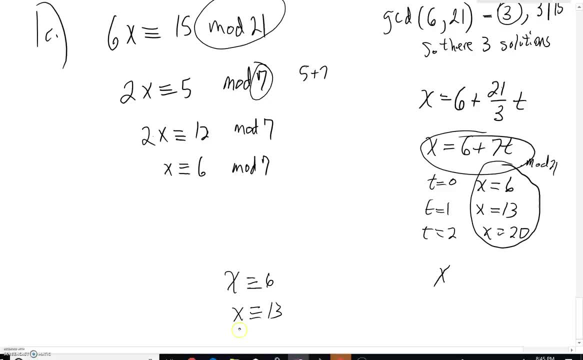 X is congruent to 13.. X is congruent to 12.. X is congruent to 20.. All of these would be in mod 21.. You know our answer previously was good. Even that's what the author did.